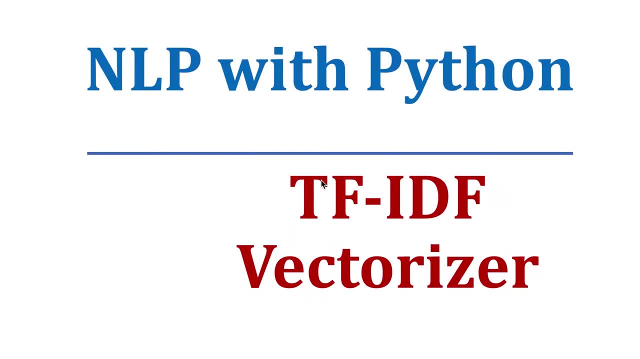 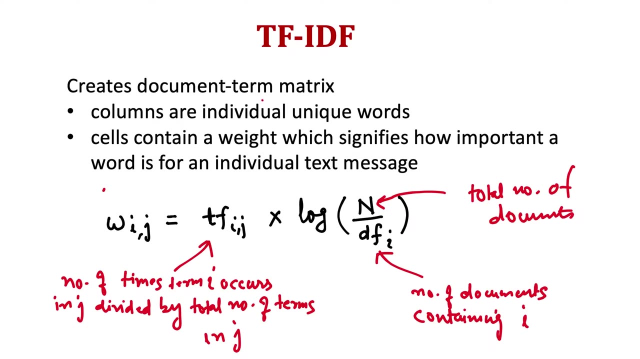 In the previous two videos we have seen count vectorizer and n-grams vectorizer. So in this video we will see another vectorization technique called TF-IDF. So it also creates a document term matrix similar to count vectorizer and n-grams. 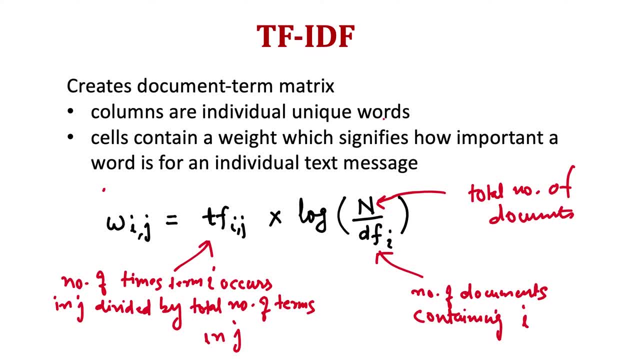 And here the columns are individual unique words, same as count vectorizer. And in n-grams we saw that columns were all the combinations of adjacent words of size n, where n will depend on what gram we are using. So here it will be unique words. 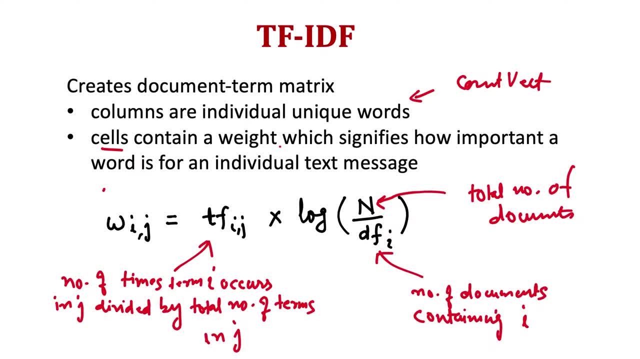 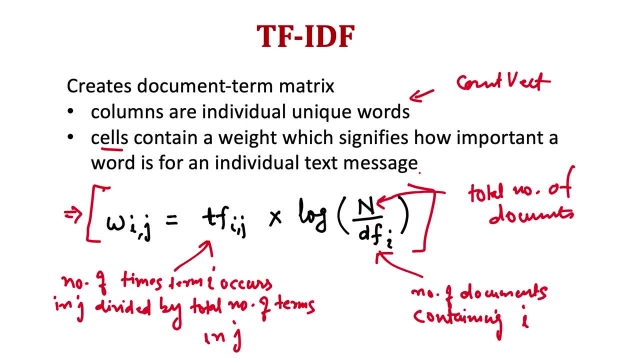 which will be calculated using this function. So in this case, it will contain a different weight, which will be calculated using this function. So in this case it will contain a different weight. word is for an individual text, message or a document, and we will see why. how is this weight? 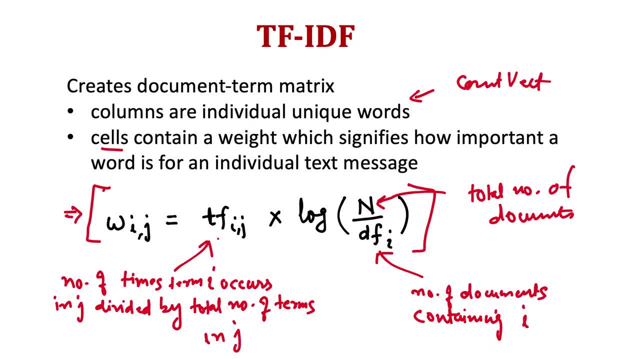 signifying that. so it depends on two things. here we see that one term is tfij, which is number of times a term i occurs in a document, j, divided by total number of terms in j. so if we have a sentence which contains five words and a word occurred two times in that sentence, then it will be two divided. 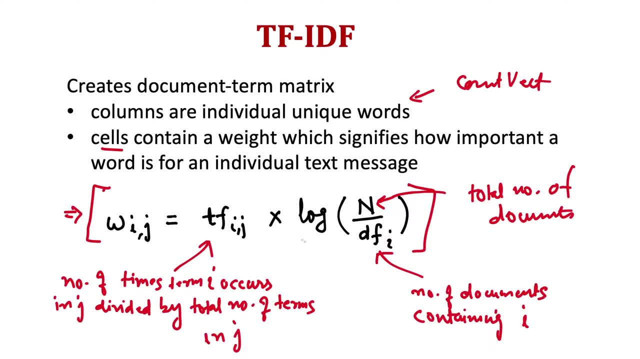 by five. and then we have that multiplied to log of n, where capital n is the total number of documents in that corpus and dfi is the number of documents which contain the term i. so let's uh. so what if uh a term occurs? so let's uh. so what if uh a term occurs in a document? j divided by total number of terms in. 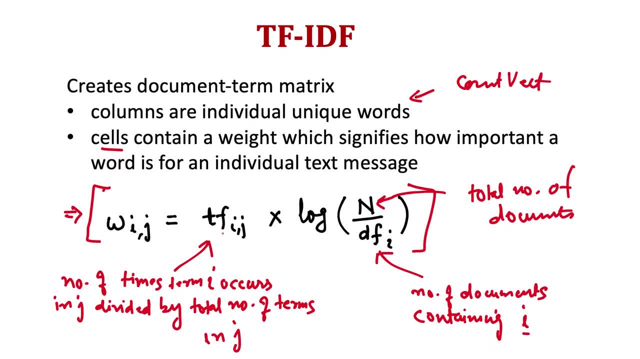 frequently in any document, then this numerator will be number of times I occurs in that document- J, so it will be high, divided by total numbers of terms in J. so that term is occurring very frequently in that document as compared to other words in that document. so it will be high if the frequency of a word 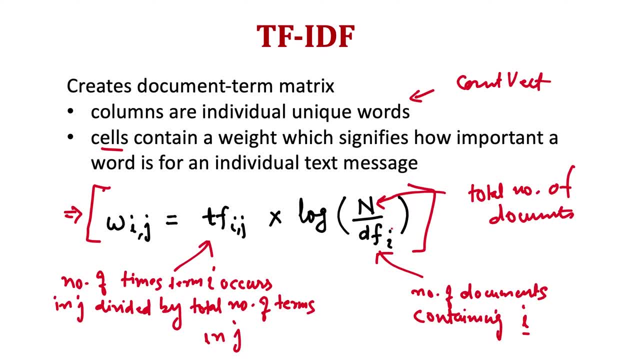 is high in a given document and this is in the denominator. so if this is a smaller, this complete term will be larger and this term denotes number of documents containing I, so if this word is not very frequent in other documents. so if a corpus has 10,000 sentences and we are looking at a particular sentence, 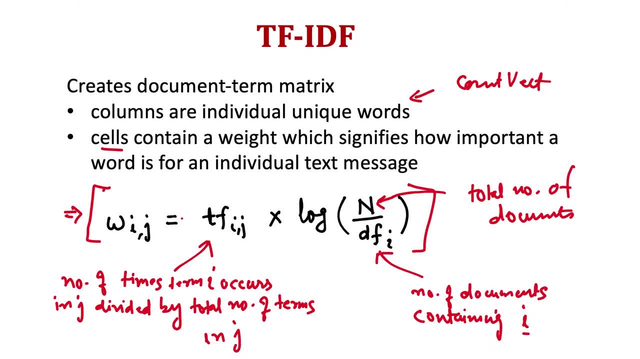 where some term I is occurring, but we see that that's not very frequent. in other terms, that means that word is rarely used, that is not commonly used. that's why it's not present in other documents. you, so it will be smaller and the overall term will be larger. so if a word appears, 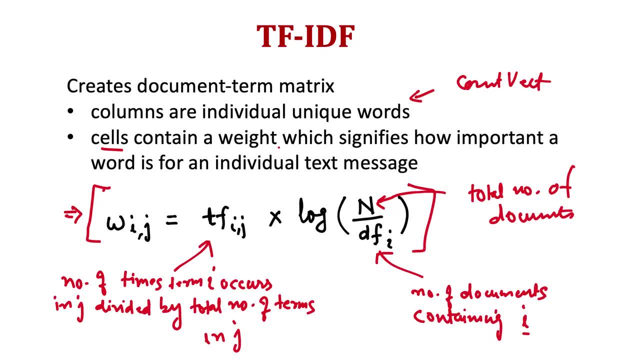 more number of times in a given sentence, but it's a rare word, then this complete term will be large. so W I, J in that case will denote how important the word I is for differentiating that document J when compared to other documents. so let's look at an example. so we are given a 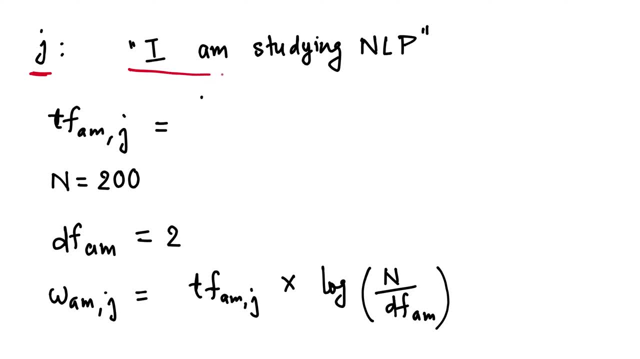 let's say, Jth document in a given corpus is this: I am studying NLP, so first we need to calculate EF of M. let's say we are calculating for this, so here I is this M, so this is occurring just one time here. so it will be 1 divided by 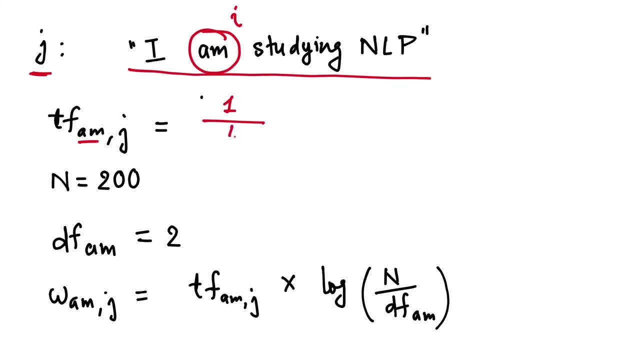 total number of words: 1, 2, 3, 4, 4, so it's 0.25. now N is 200, so this corpus contains 200 documents. we are given this and D F of M is 2, so BS denotes number of documents containing I. so it denotes that out of those 200 sentences, 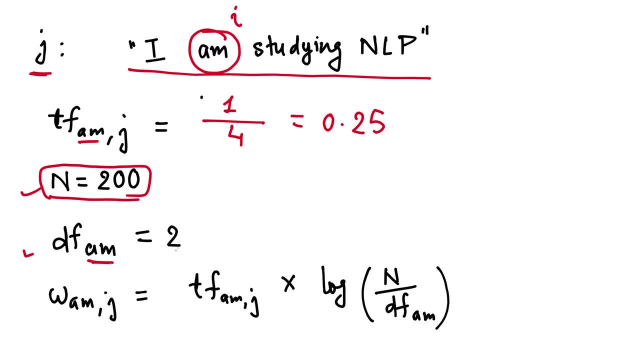 or documents only its present in two sentences, so it's quite a rare word for this corpus. so now let's calculate the W AMJ, which will be the value of cell in document term matrix. it's 0.25 and multiplied by log of n is 200 and df am is 2, so this will be 200. 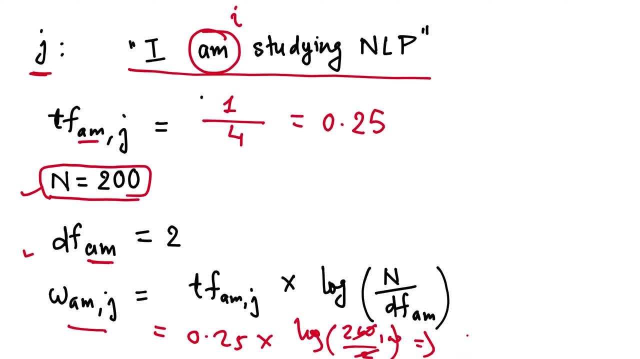 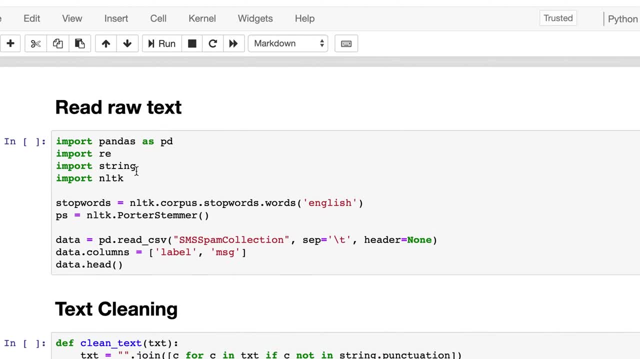 divided by 2, which will be 100, and log 100 will be 2, so it will be 0.5. so now we are ready to write the code for this, so it will be very similar to our count vectorizer code. so the first part is: 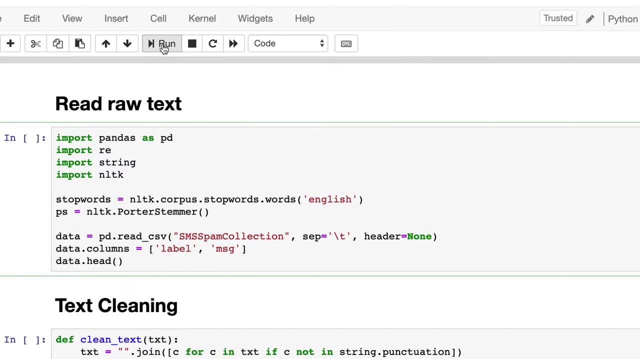 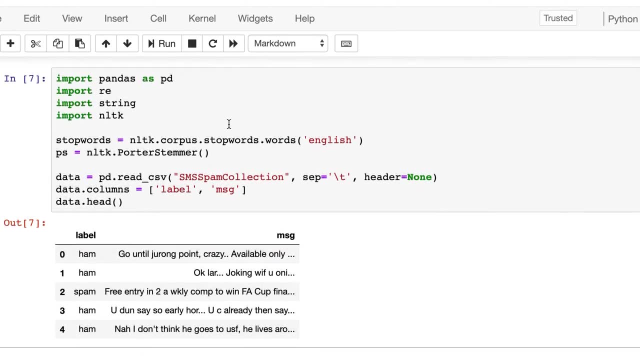 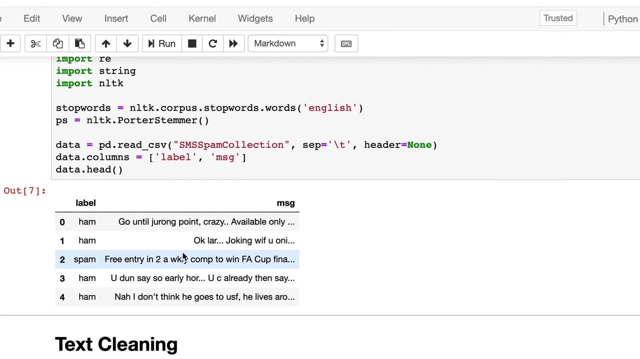 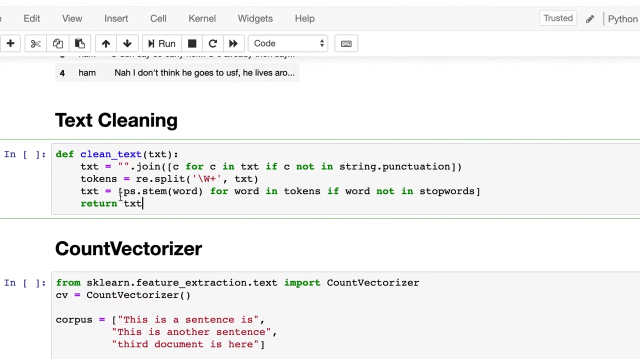 reading the raw text, which will be same as count vectorizer. so let's run it and here we are, dividing the data frame into two columns: one is the message and the second is the label containing ham or spam. and then the text cleaning part will also be same as count vectorizer. in the n grounds: 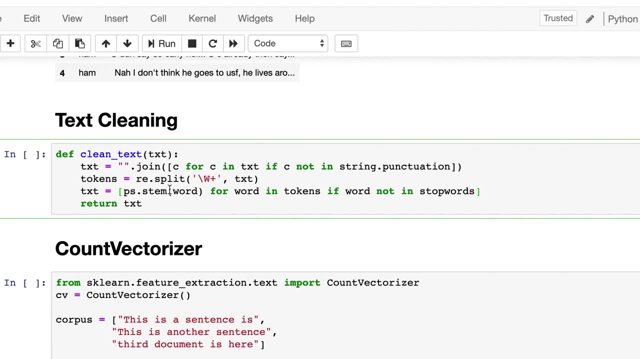 we had modified this text, cleaning slightly and we were joining a the words clean words, after removing stop words, the list containing those clean text. we were joining into sentences separated by spaces, because n gram expects sentences so that it can look at all the n adjacent words in the documents. but here we don't need to do that. here the columns. 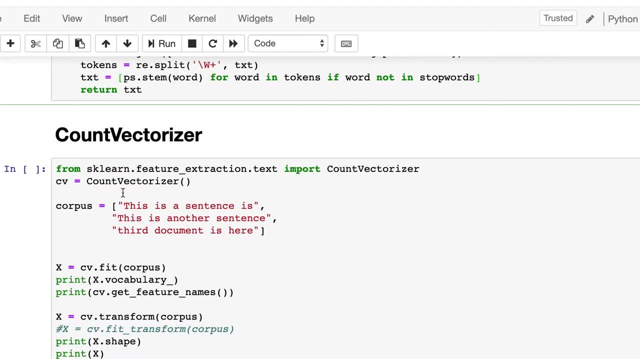 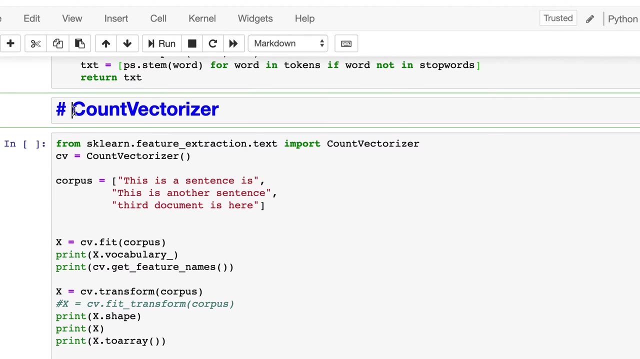 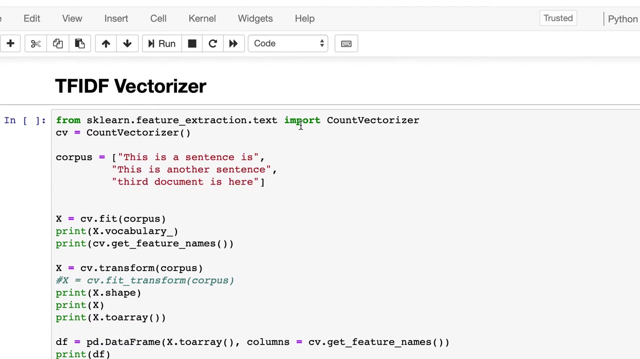 exactly is same as count vectorizer, only the cell values represent a different weight, whereas in the vectorizer the cells represented the frequency of a given word in a particular sentence. so instead of count vectorizer, let's change it to tf id of vectorizer, and it will also be present in this. 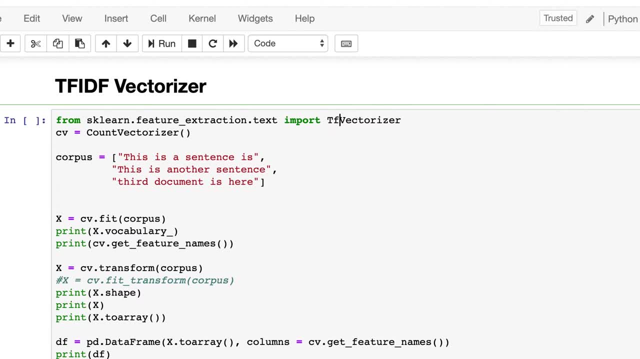 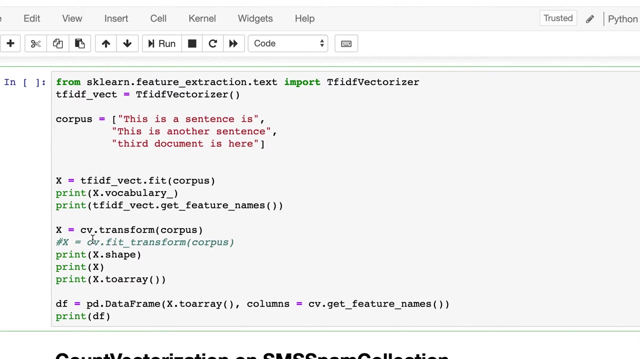 sklearn feature extraction dot text. but it will be tf id of vectorizer and let's create an instance of that and call it tf id of vect. and this is our dummy corpus which contains three documents. so we are fitting the tf id vectorizer on this, so it will create a vocabulary. 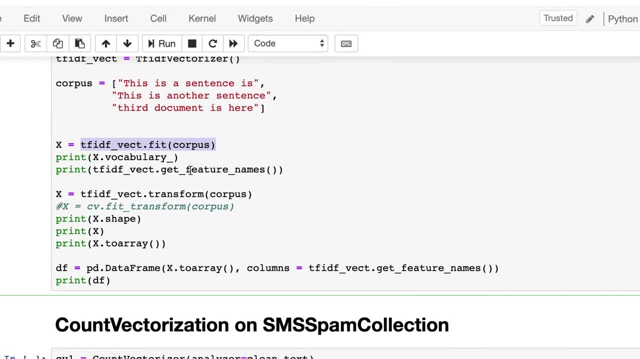 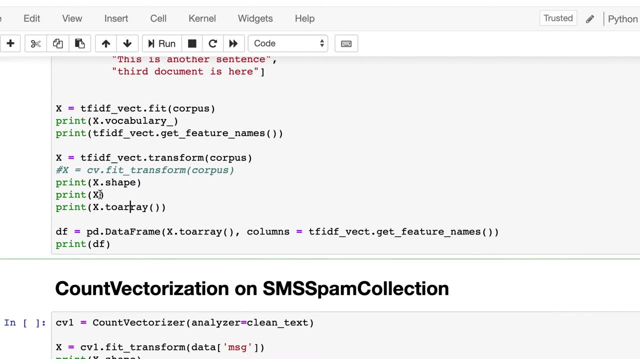 but it will still not calculate the tf id of values when we do translation of the text. so let's create a vocabulary and let's call it tf id of vect transform. it will do that and create the document term matrix. and this is a sparse matrix because 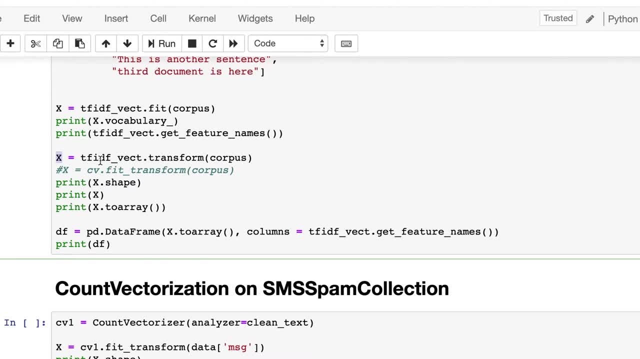 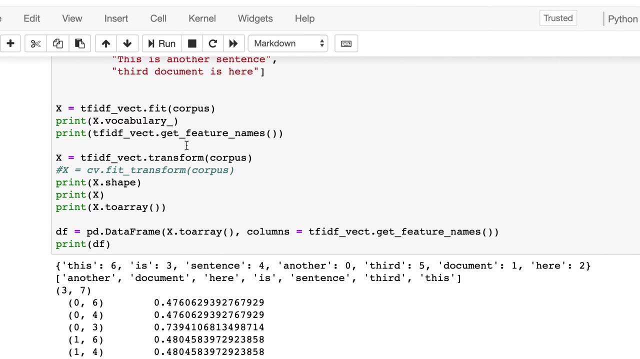 most of the terms are zero, so by default it will be a sparse matrix and then when we want to convert it to data frame, so doing this two array it will convert it to a full-sized matrix and then we can create a data frame out of that and print that. so let's run it. we see that these terms, the columns, 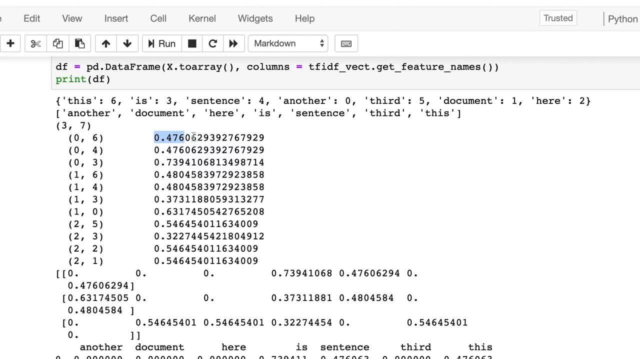 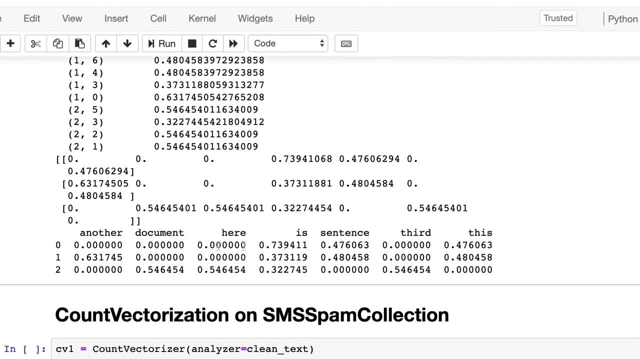 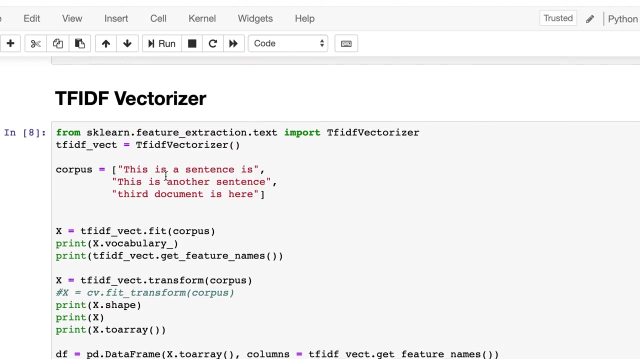 are exactly same as count vectrider and these are the individual values. so the same as what we had calculated in our example. and this is the data frame which contains the tfяд of values for each word in a given document. so now let's do the same thing for our sample or data set. so again, let a. 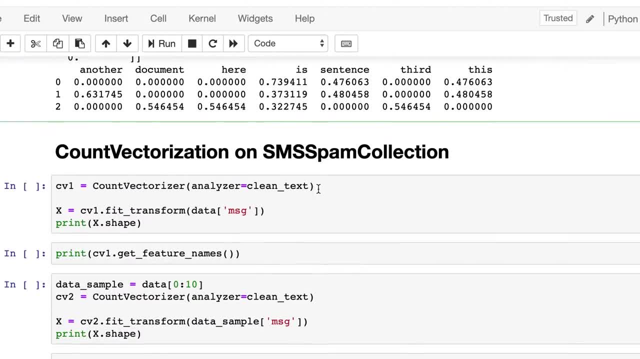 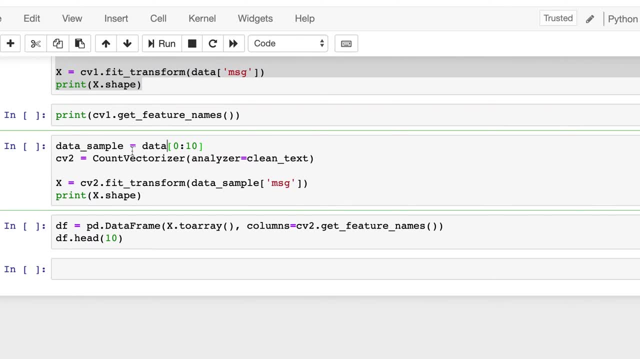 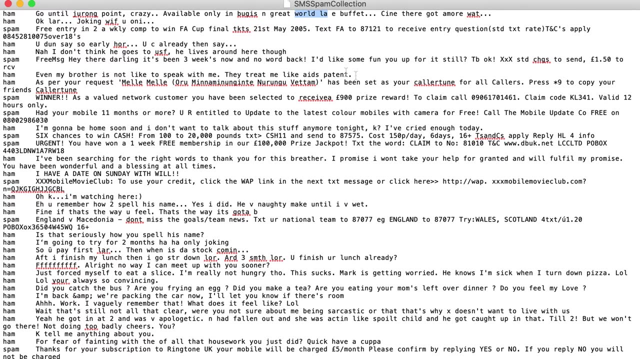 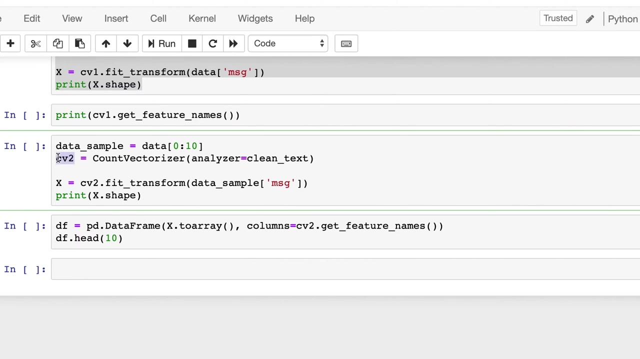 table III de laث x. So let's just skip this part. This is doing on the complete corpus, which will be too big. So for our case, we will be picking up first 10 messages from this SMS spam collection data set And let's name it tfidf2, and it will be here: tfidfvectorizer. 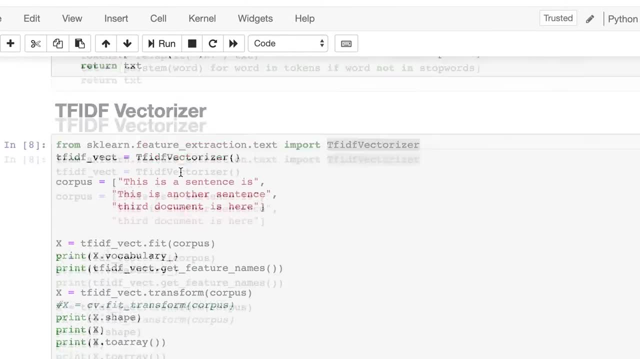 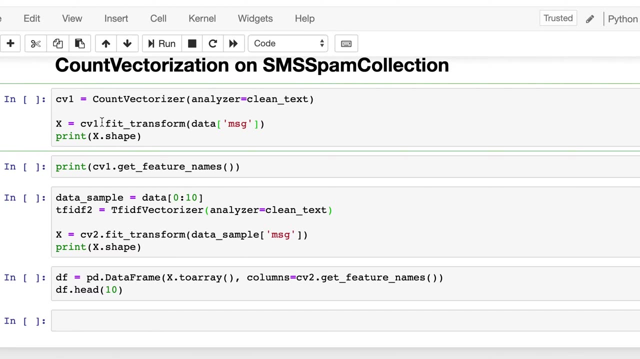 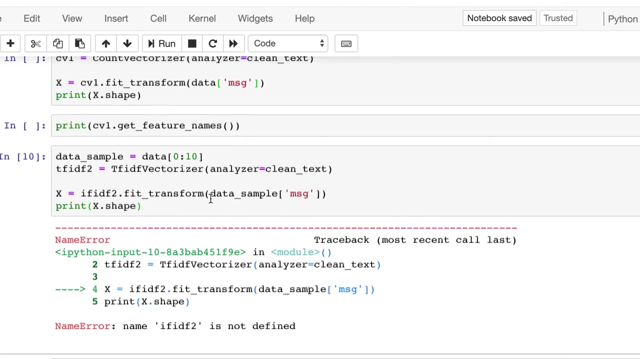 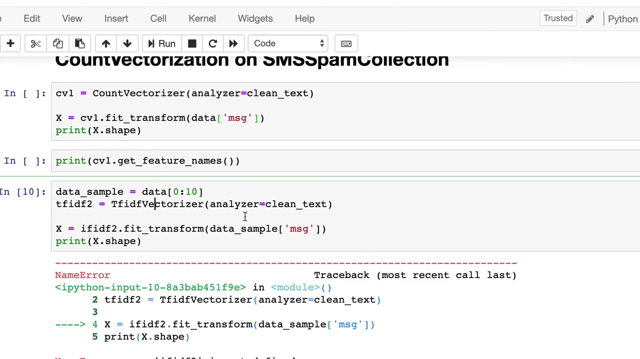 And we will pass here our cleantext function. So we have not run it. so let's first run it, And then we will call the fit transform on this tfidf2.. Let's run it, So it says tfidf2 is not defined. 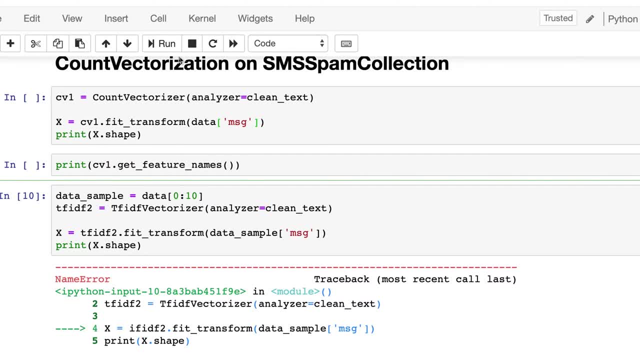 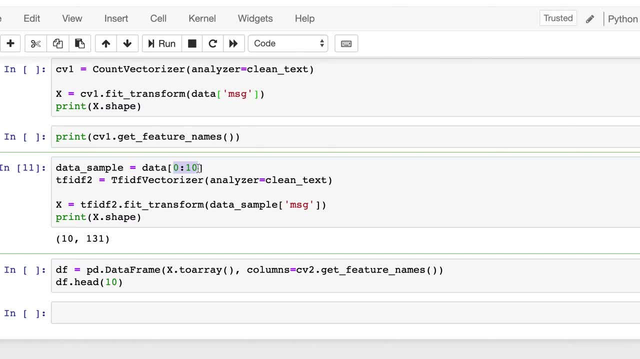 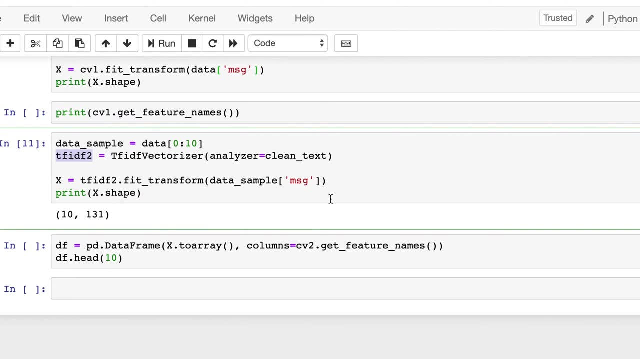 OK, there is a typo here. So now it has 10 rows because we had selected 10 rows of the entire data set And it has 131 columns. Let's print it. Let's print the data frame, OK, OK.